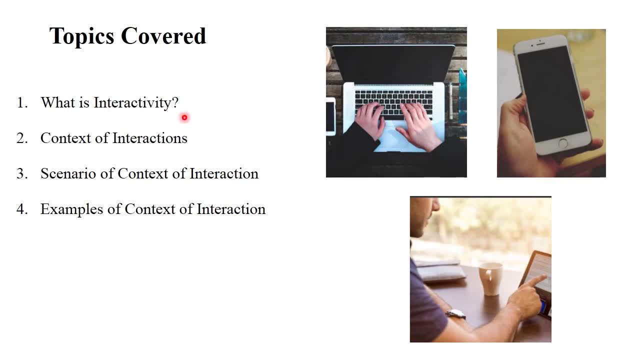 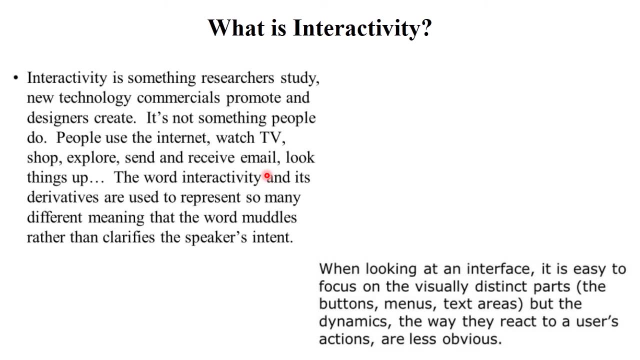 So let's see one by one. The first one is: what is meant by interactivity Next, So interactivity is one of the simple concept. In our daily life, or in our real life, we always use interactivity, interaction, these kind of concepts. 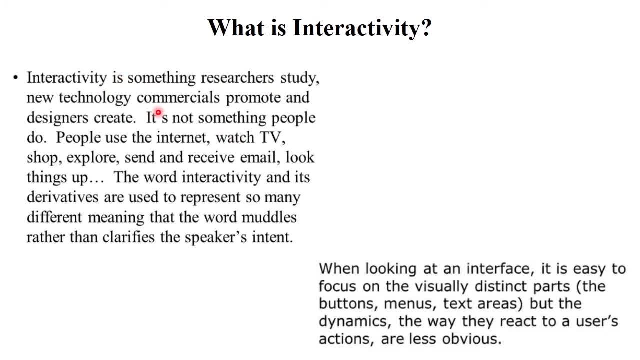 So interactivity is something researchers study, a new technology commercial promote and designers to create. It's not something people do. People use the internet: watch, TV shop, explore, send and receive email and do things up like this. 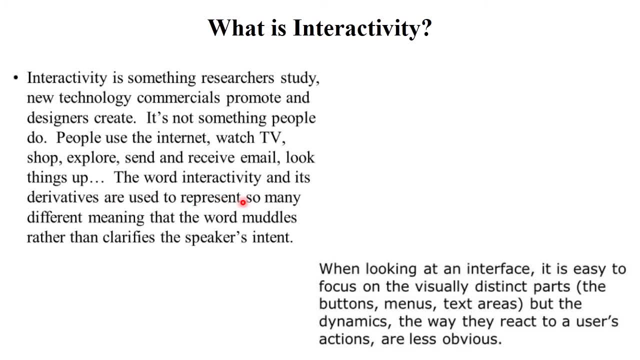 The word interactivity and its derivatives are used to represent so many different meanings that the words models rather than clarify the speaker's intent. So simple interactivity means how users are interactive with different types of technologies according to different features or specifications of that particular applications. 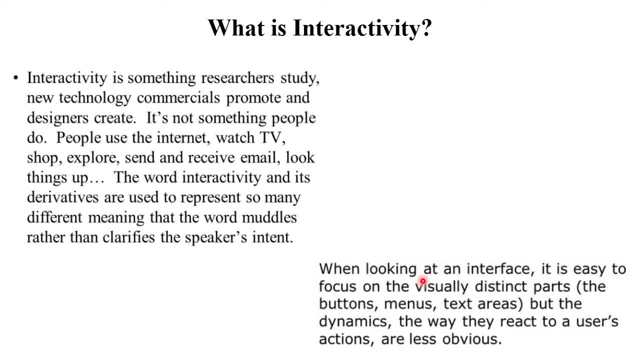 So again, interactivity simply means when looking at a particular interface, it's easy to focus on the way the user is interacting. So again, interactivity simply means when looking at a particular interface, it's easy to focus on the way the user is interacting. 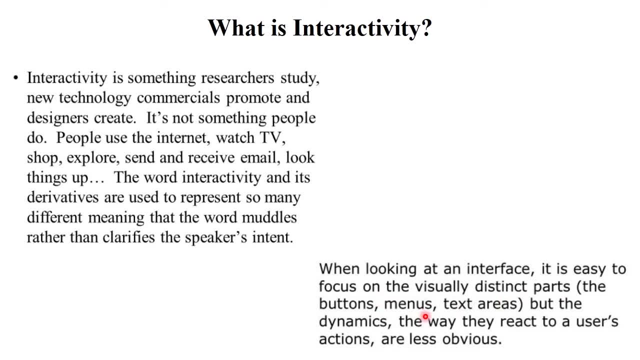 And there are not only visually distinct parts like buttons, menus, text areas, But the dynamics, the all are dynamics, or, as per our requirements, we have to use these kinds of features, So the way they react to the user's action are less obvious. 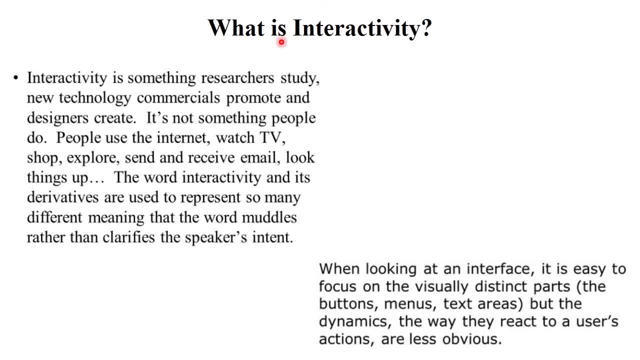 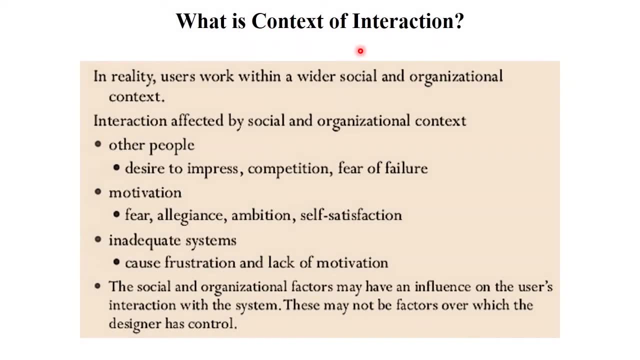 So these all kinds of concepts are included in the interactivity here. Next Now the context of interaction. So context include only three types, like other people: motivation and inadequate system. in reality, users works within a wider social and organizational context, right, so interaction affected by the social and organizational 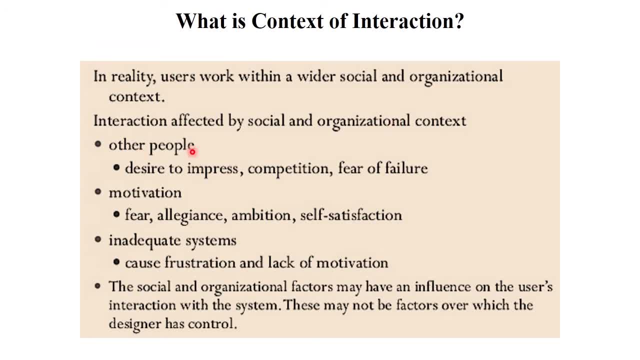 context, for example, other people as per other people, we desire to impress. competitions, fear of failures- this kind of context are included in our daily life, means we used a particular technology or we develop a particular technology by competition or desire to impress other, our users, right. the next one is motivation. motivations means we 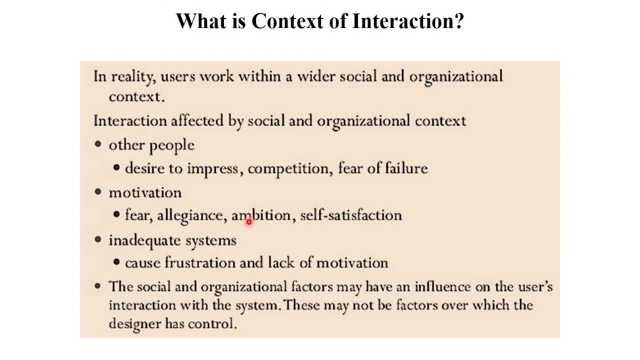 motivated, which includes the fear, elegance, ambitions or self-satisfaction- right. so as a developer, developer develop a particular product. this is just ambitions, right. the next one is inadequate system. inadequate system includes the cause: frustration and lack of motivations. some systems have bad user ID or a bad design. 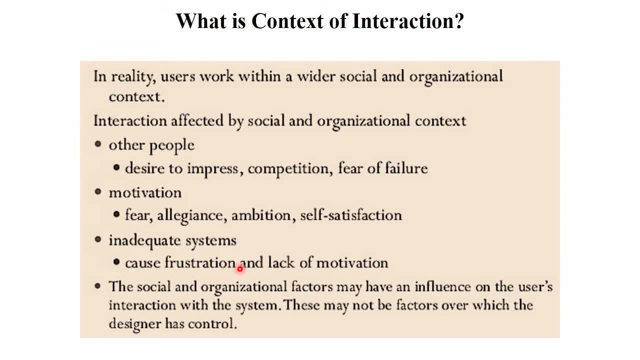 okay, so it caused the frustration and lack of motivation to the developers as well as users. so the social and organizational factors may have an influence on the users interaction with the system. right, as per our requirement, as per our organization, we use particular technique among particular technologies, right, so these may not be factors over which the designers has control it. 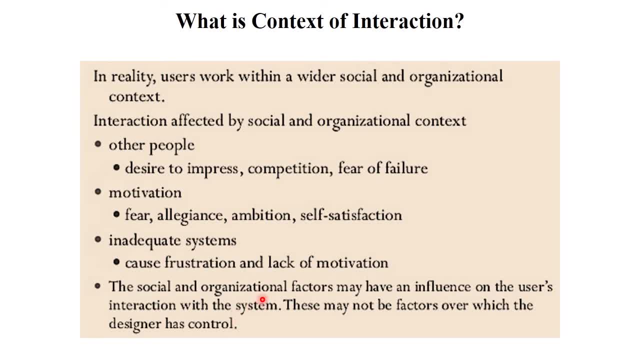 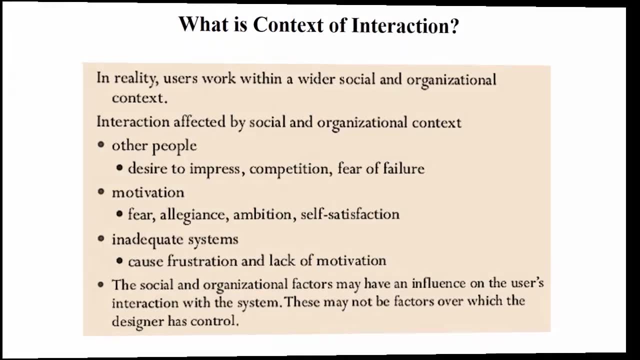 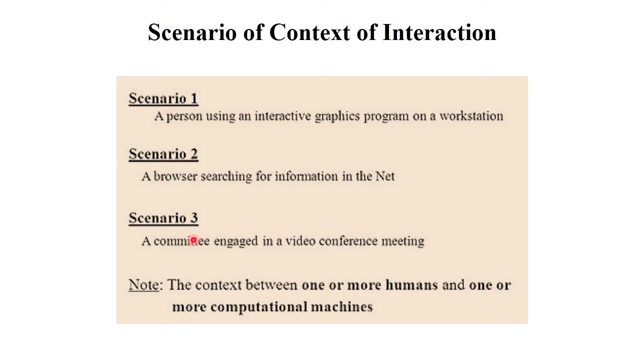 completely depends on our work, our organization and our social behaviors clear. so these are the context of interaction. next, the next topic is scenario of context of interaction. see here there are some scenarios. first scenario is a person using an interactive graphics program on workNet station. There are different websites or games have a particular interactive graphical interface. 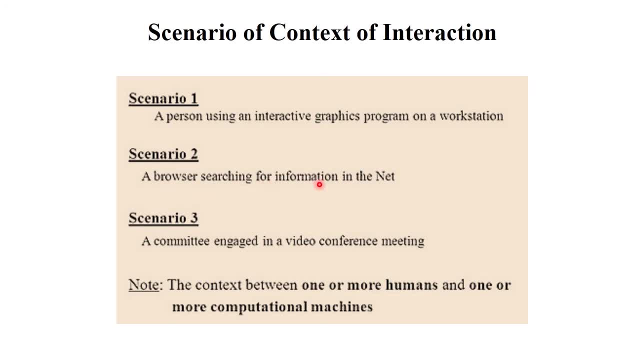 right. The next scenario is a browser searching for information on the net. We use different types of browsers for searching information. right. And the next scenario is a committee engaged in video conference meeting. There are multiple workers are used video conferencing app for meeting right. 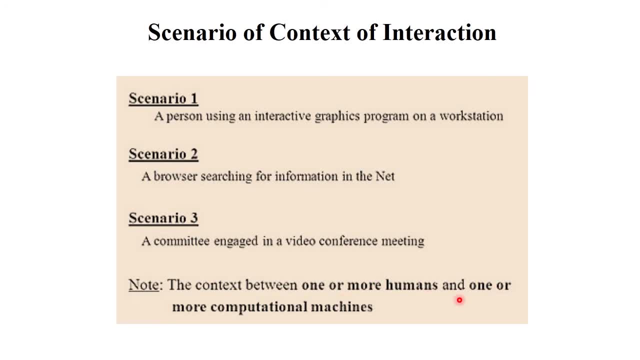 So the context between one or more human and one or more computational machines. It's called as context of interaction, right So context means simply the particular technologies, techniques, how these users are used, that particular applications, right So these are called as context of interaction. This is generally between one or more humans or one or more computational. 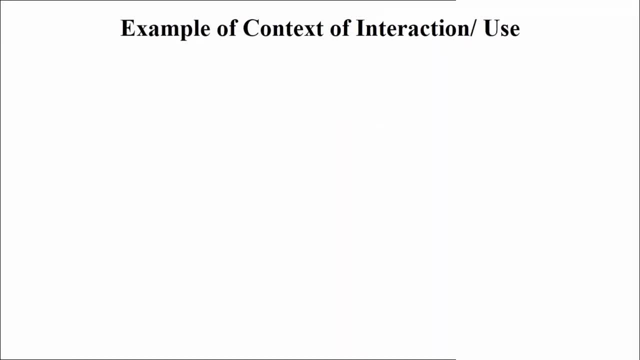 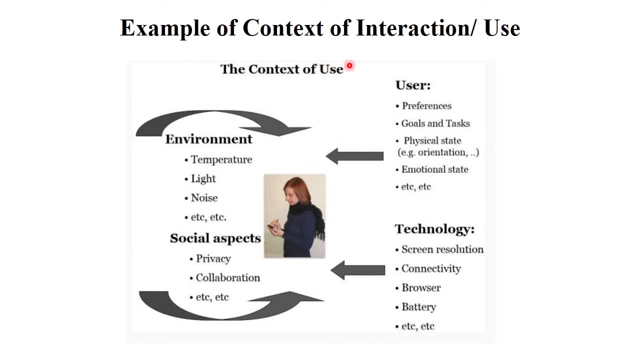 machines Clear Next. Now again next example of context of interaction. So see here The context of use. There are total four areas like users, technology, environment and social aspects. right, So what is the context of users? Users have their own preferences, own goal and own task. right, User used a particular.